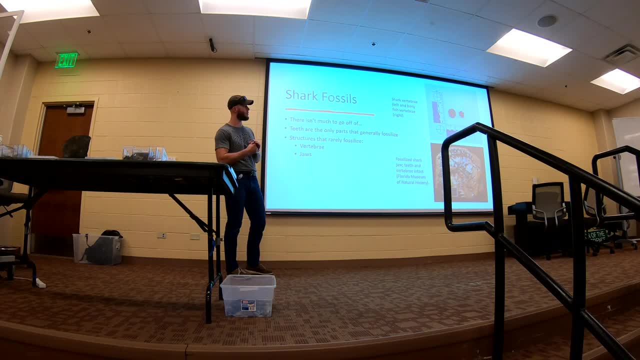 that fossilize. That top picture on the left that's a shark vertebrae and right next to it is a bony fish vertebrae. Those are pretty rare to come across when I was doing my research And jaws rarely fossilize. This is like a really rare specimen from the Florida Museum. 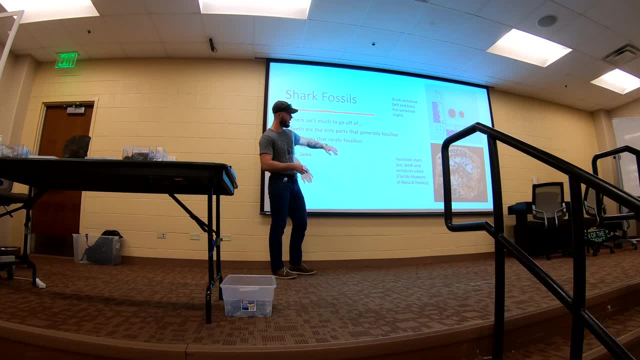 of Natural History. You can see that the upper and lower jaw is there and the vertebrae are there. So you can see that the upper and lower jaw is there and the vertebrae are down at the bottom, with all of the teeth intact. That's really rare for that to happen. 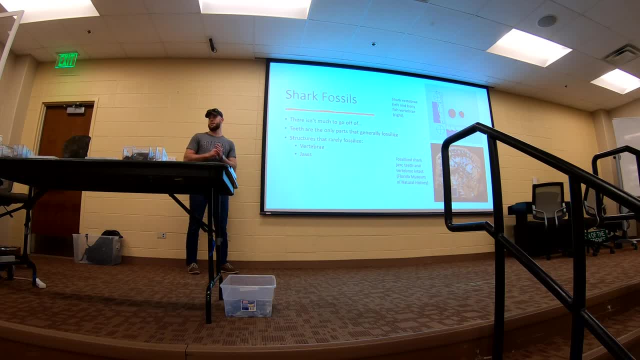 So really the only thing we have to go off of are their teeth, And that can pose a lot of questions, like when we're trying to reconstruct a megalodon: We don't really know what it looked like. We know what its teeth looked like, but we can't really have an accurate representation. 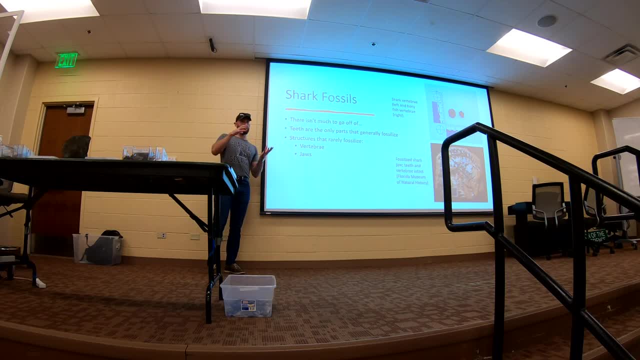 If you see, like the movie The Meg and stuff, it's basically like a blown-up bright white shark And it's not. we don't know that for a fact because we don't have any fossils up there of their fins or their backbone or anything like that, so it's tough to tell. 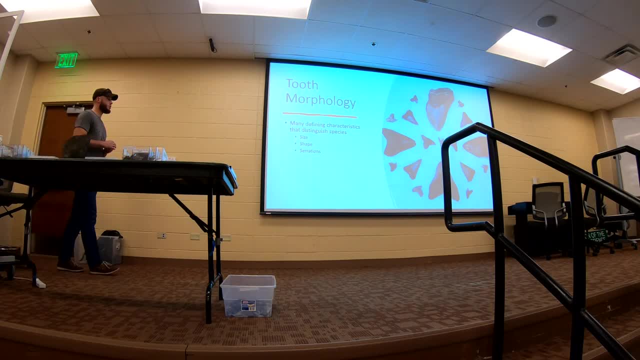 a lot about sharks just from their teeth. A little bit about tooth morphology. They vary greatly from species to species. As you can see here. there's lots of different species in that photo and they can vary in size, shape, serrations and a lot more. So the 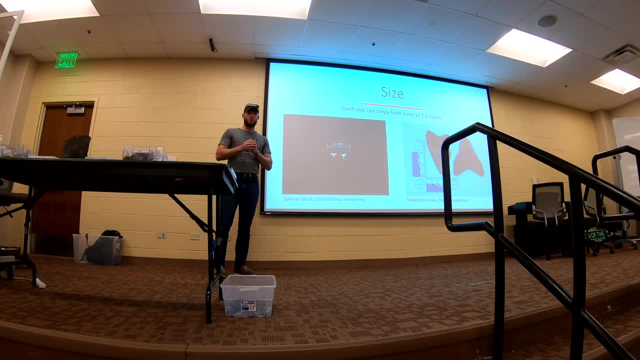 first thing is size. Tooth size can range quite broadly. So these these, uh, these These teeth here were loaned from the Fordham Museum of Natural History for this study, And this is from a spinner shark And you can tell that from the scale. just one centimeter teeth can be really small. 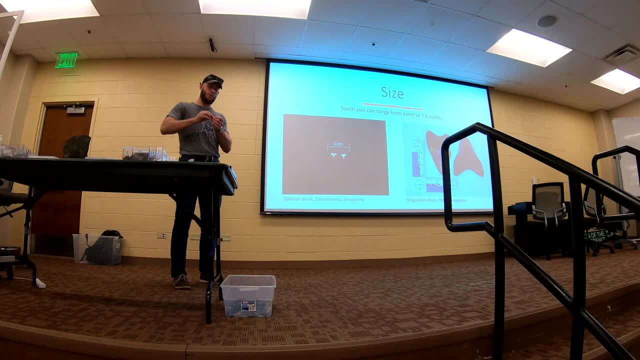 They can just be a couple millimeters big, So you guys probably can't even see this tooth right here, But they can also get really really big. like this. They get really big, And this is 5 1⁄2 inches, and the largest megalodon tooth ever found was 7.5 inches. 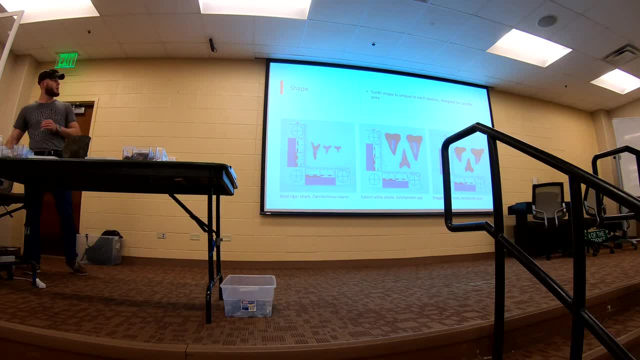 Shape. Okay, so tooth shape is unique to each species and they're designed for a specific prey. So on, here we have a sand tiger shark, And while their teeth look pretty jagged, you know, they have these little side teeth. 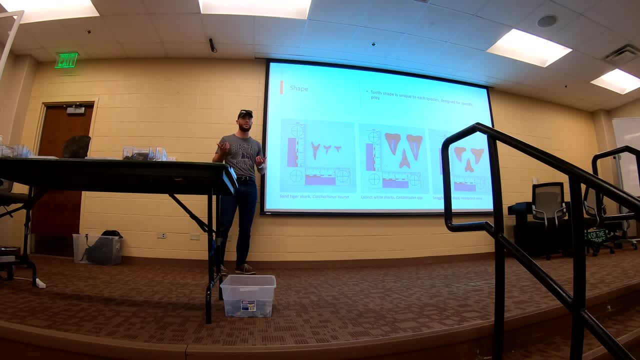 they look kind of ferocious when you're looking at a sand tiger shark, But there haven't been any recorded bitings from sand tiger sharks because their jaws don't open very big. They keep their jaws just open so slightly that fish can swim inside. 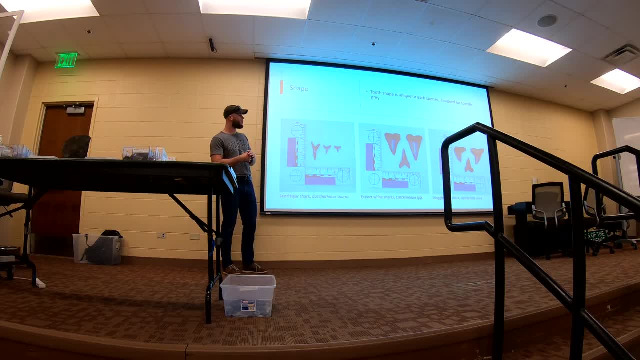 And they can get caught in their jagged teeth. Over in the middle we have the extinct white shark, so the predecessors to the great white. You can tell. their teeth are much more triangular And if you notice that tooth that's facing upward, that's a lower tooth. 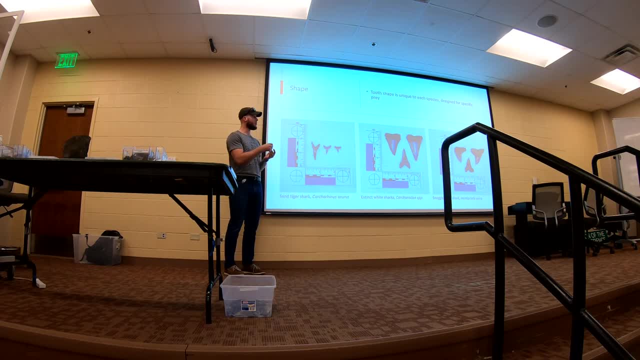 The lower teeth on sharks are a lot different from the upper teeth. The lower teeth are more slender and peg-like, And what they do is they kind of act like stakes that you would use for a tent, And they keep the prey in place, while the upper teeth do most of the thrashing. 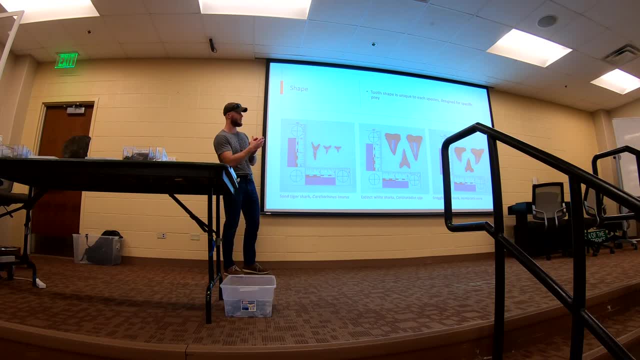 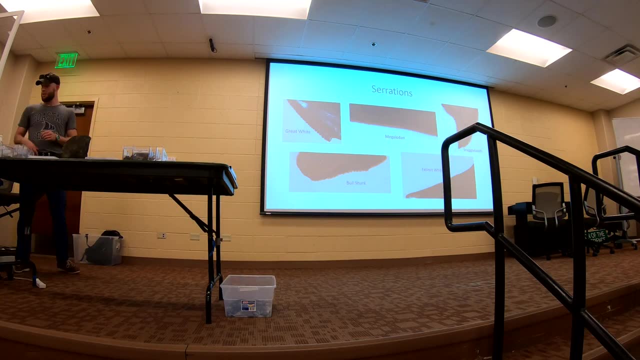 And on the far right you have a snagletooth shark, a really pretty shark that has a distinct curve and really jagged serrations. So some more serrations. You can distinguish species just by their serrations. So in the middle up top you have megalodon serrations that are really fine. 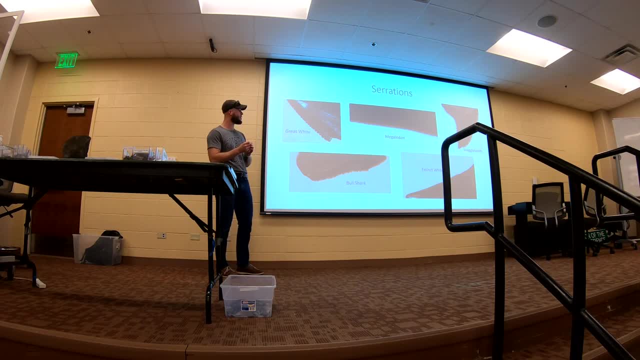 Each serration basically looks like the next one, the one next to it. Great white serrations are much different than megalodon serrations. You can tell that right here, and right here those are called complex serrations, Where one serration just kind of breaks off and it's like one serration that's kind of fused with another. 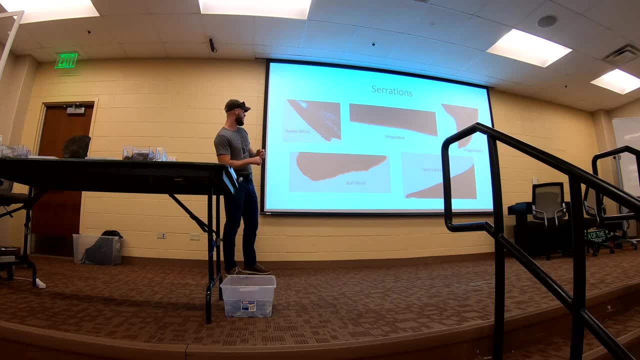 Snagletooth serrations. you can see they're pretty jagged. And bull shark, you know they're very irregular, they're very plump, Each one is different from the next. And you also have teeth with no serrations, like the extinct white sharks. 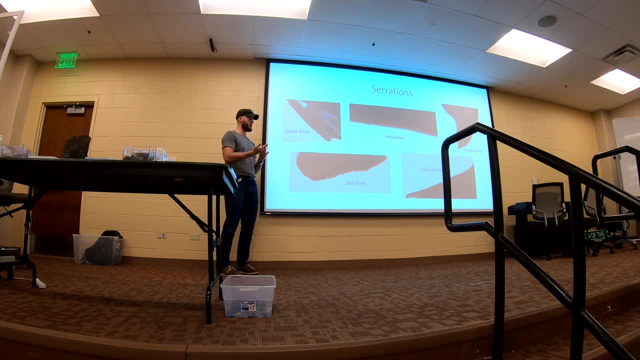 And if you look at an extinct white shark and the modern great white shark, you can see that the only difference between the two was that the great white shark developed teeth And the new white shark developed serrations over time. Alright dentition. 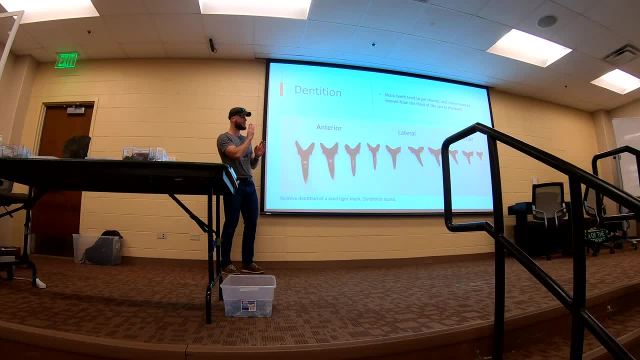 So the dentition of a shark or how the tooth is positioned inside the jaw, Each tooth is different. As you move towards the back of the mouth, each tooth is different, Just kind of like how our teeth are. Our front teeth are different from our back teeth. 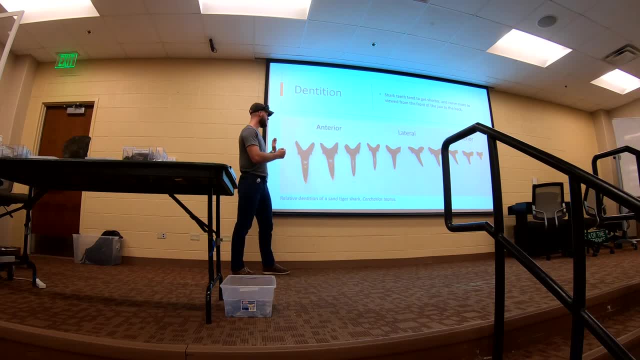 So if this is the front of the jaw and we're looking towards the back, you can tell, you can see that the teeth slowly get smaller And these tend to curve a little bit more. So we call the front teeth the anterior teeth. 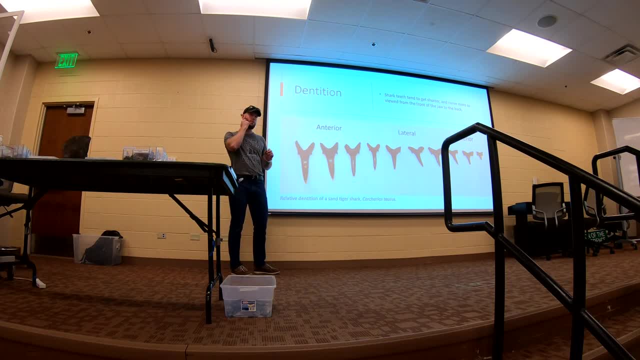 The side teeth and the side of the jaw, the lateral teeth And the very back, the posterior teeth, And so basically across all sharks. their teeth tend to get shorter and curved more as you move towards the back of the mouth. So that is the relative dentition of a sand tiger shark. 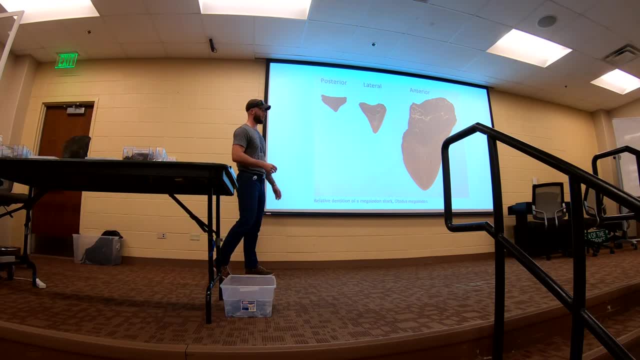 And this is the dentition of a megalodon shark. So you can see. the one on the right is an anterior tooth, the front tooth, And then on this, as you move towards the back of the mouth, this is the anterior tooth. 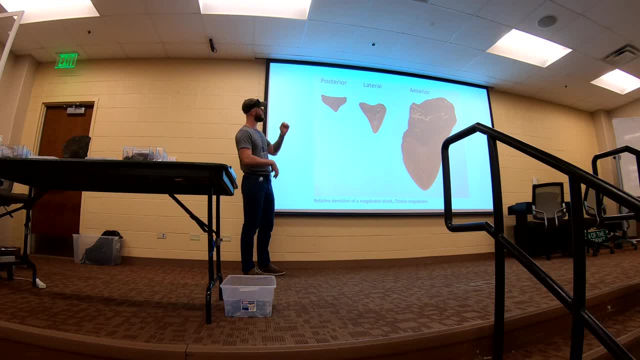 And then on this, as you move towards the back of the mouth they start to get more curved And that's the lateral tooth And the posterior tooth is really stubby. So when you hear some people talk about megalodons and they say 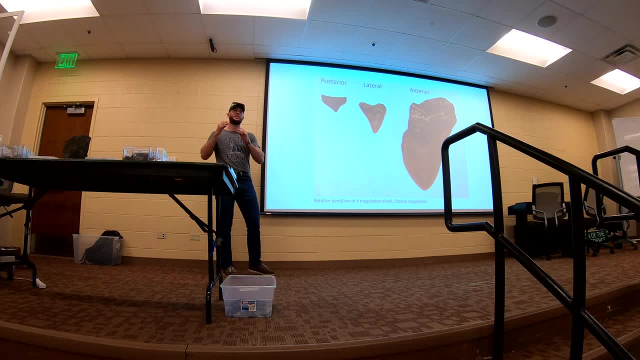 well, they had 256 teeth at once and they were all 7 inches. That's not the case. You know, they get smaller as they go towards the back of the mouth. So technically, like that tooth on the far right and the tooth on the far left. 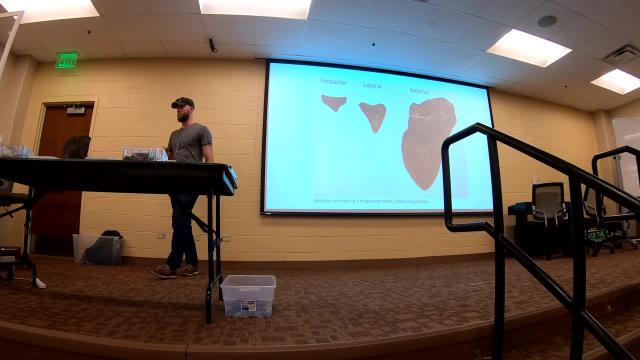 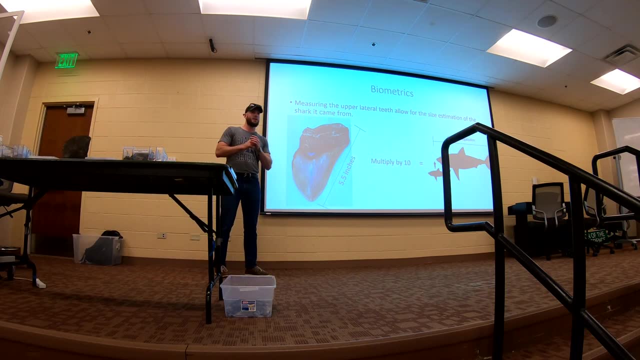 those could technically be from the same shark. They just get much smaller as they move towards the back. Biometrics: I learned about this with Dr Demi in his Coastal Research Methods class on Sapelo. Basically, what we can do is if you have an upper anterior tooth. 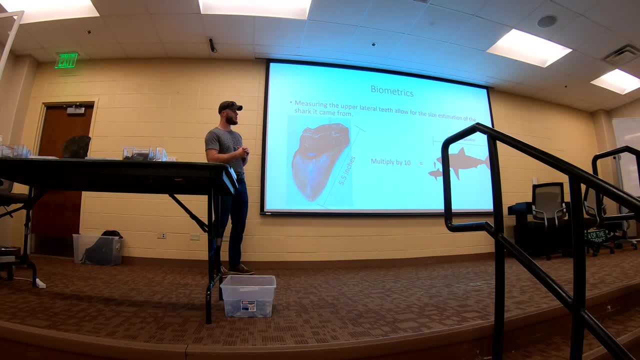 so upper tooth and towards the front of the mouth, you can measure the tooth and estimate the size of the shark. So my largest specimen, this megalodon tooth, if you measure from here to here we get 5 1⁄2 inches. 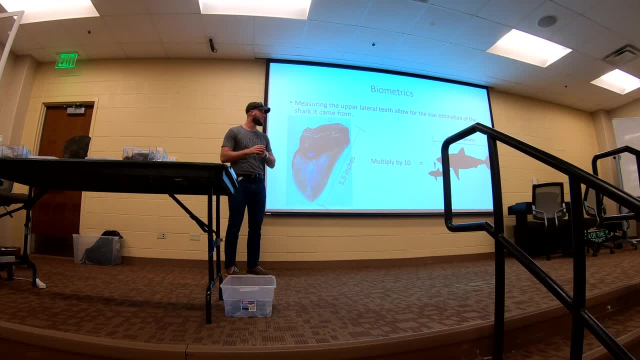 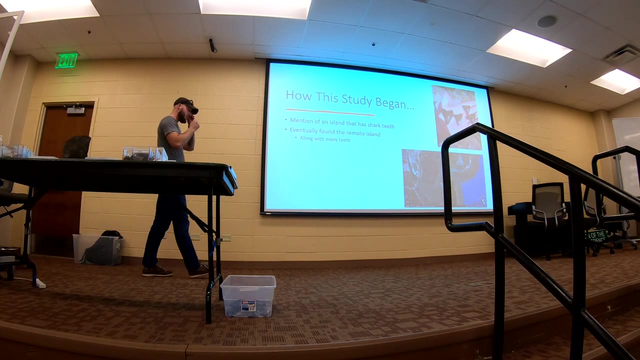 And you just do a simple conversion: You multiply it by 10. And that equals a 55-foot megalodon. So for comparison, great whites don't get past 20 feet, So it was a big shark. All right, So entering into this study, I had heard from some friends 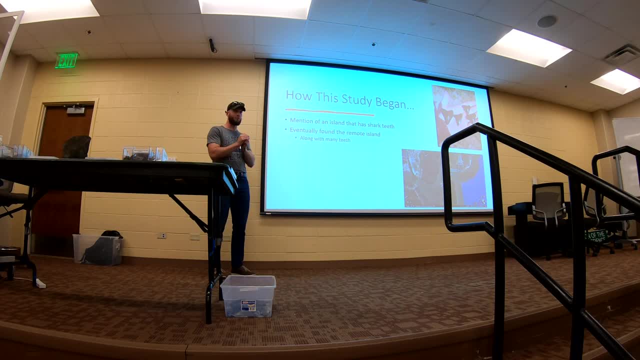 that there was kind of a remote island around Brunswick. It had really big shark teeth And so they didn't tell me where it was because it's kind of like a secret spot. So they said you have to go find it. So they said go underneath the Sydney Linear Bridge. 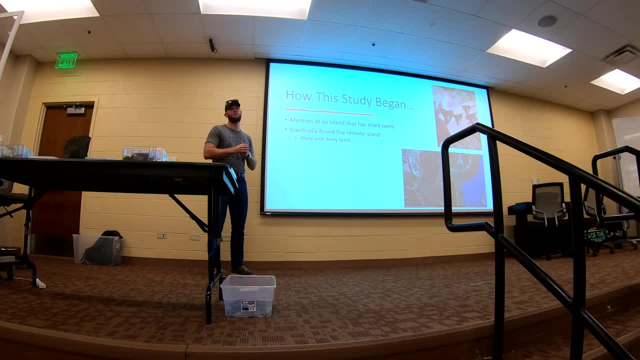 That's where you'll start Good luck. And so, after a few months, I found their little island And I started picking up lots of teeth- anywhere from 50 to 200 every time that I would go, And every with new tide, more teeth would come up. 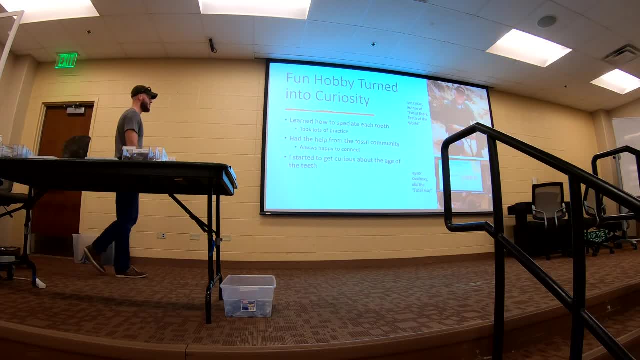 That's not the right one. Okay, So I started to learn how to speciate each tooth. I wasn't too into it at first, But then, after getting you know a good collection going, I started to realize how different the teeth were. 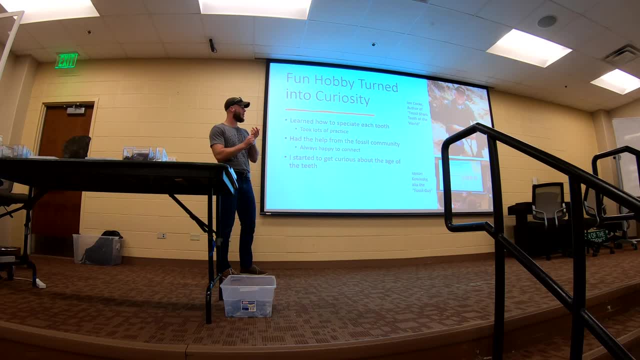 So I learned how to speciate them. I was able to talk to some paleontologists: Joe Koch, author of Fossil Shark Teeth of the World, and then a popular blogger named Jason Kowinski, also known as the Fossil Guy. 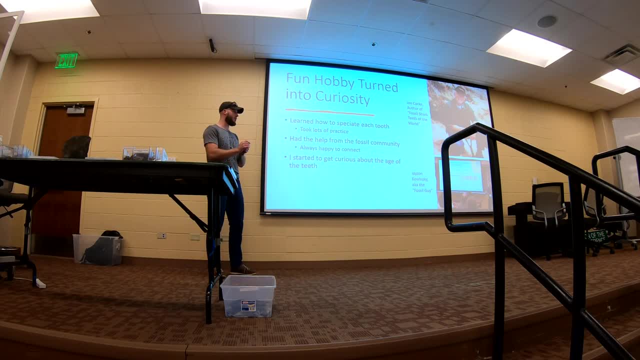 They were very helpful in helping me learn how to speciate teeth and, you know, figure out the different morphologies, And so I started to get curious about the age of the teeth. I didn't really know where when they came from. 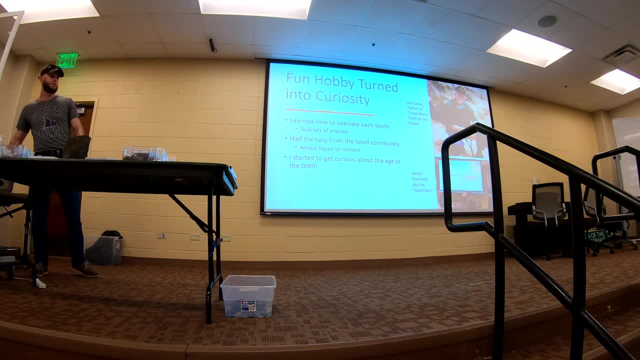 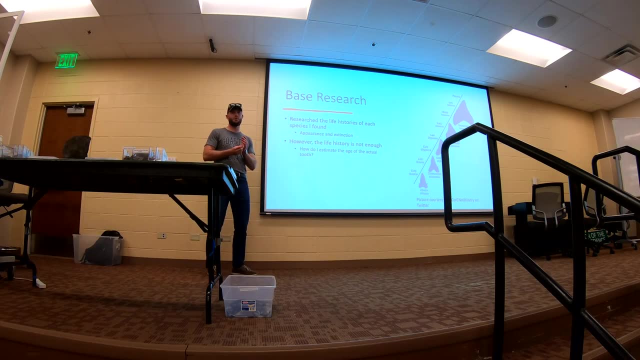 So that was slowly kind of turning the gears in the study. So I did some base research. I figured out the life histories of each species that I had found, So their appearance when they appeared in the fossil record and when they died out, if they died out. 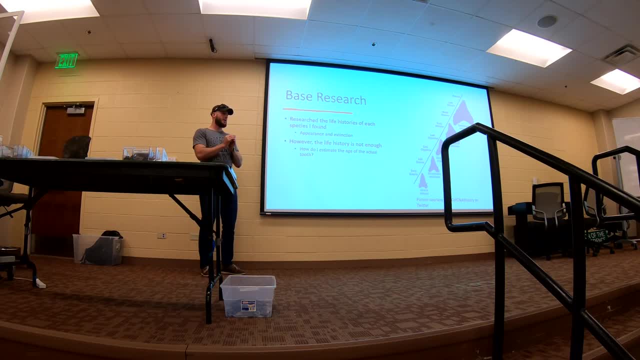 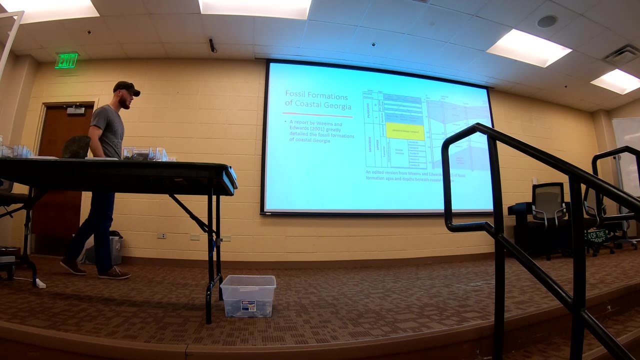 But figuring out the life history isn't enough. I still don't know when in that time period I was finding that one too, So I wanted to estimate the actual age. I wanted to estimate the actual tooth that I had, not just the age of the shark in general. 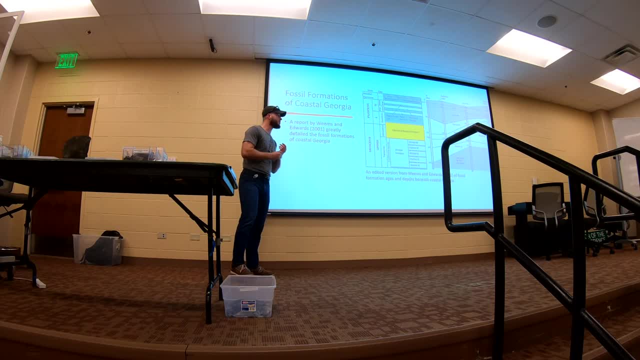 So I did some research and I found a report of someone who had mapped the fossil formations underneath Brunswick. And you can see, on the right there we have Brunswick here and this is sea level, right here, in this dotted line, And you can see the feet below sea level. 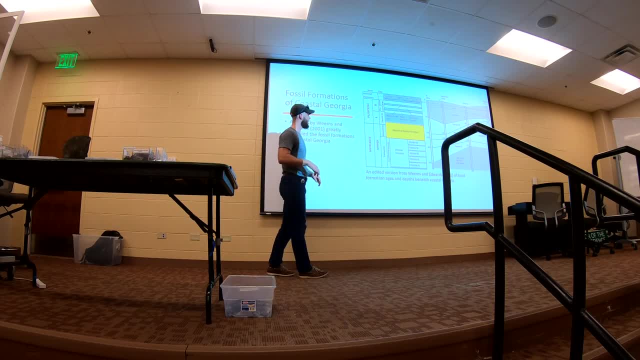 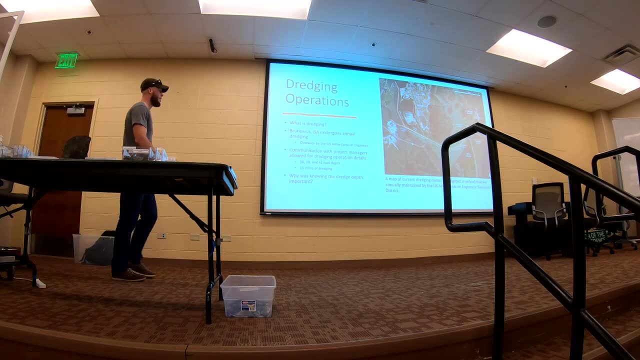 where each fossil formation was, And so that was a good start, And I was able to get the relative ages of each fossil formation. So the next step was to figure out about the dredging operations that go on in Brunswick, If you're not too familiar with dredging. 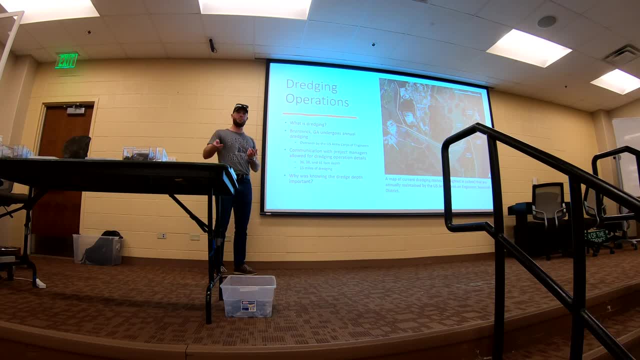 it's basically underwater excavation. We use it so that big boats can come through our intercoastal waterways because they're very shallow So they have to dredge canals. They have to dredge canals for boats to get through. 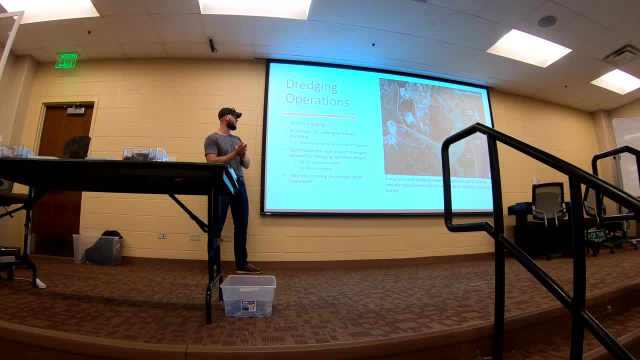 Brunswick, Georgia, undergoes annual dredging. It's overseen by the US Army Corps of Engineers, And so I was able to talk to their project managers and get their dredging operations details. They were really helpful in understanding that I was trying to do some research of my own. 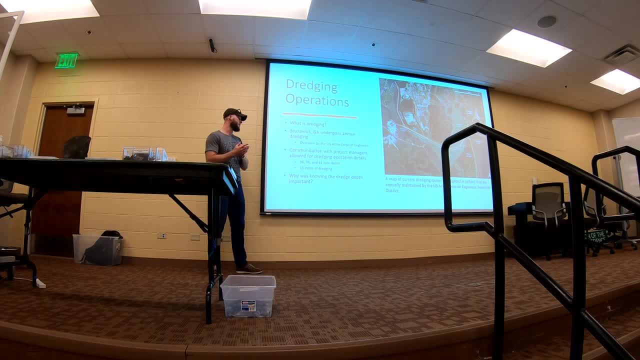 And so I figured out that they were dredging to 36,, 38, and 41 feet deep, And they had about 15 miles worth of dredging in Brunswick, Georgia, And so, knowing the dredge depth, I could now look at the map again. 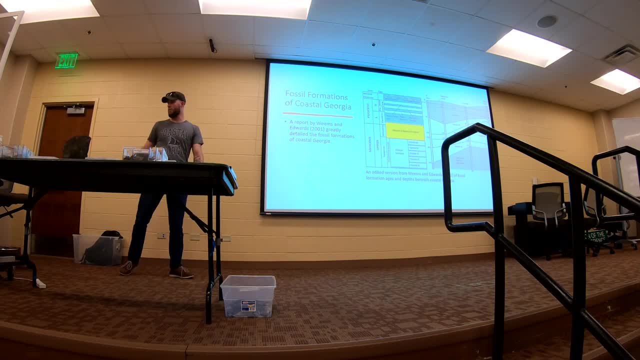 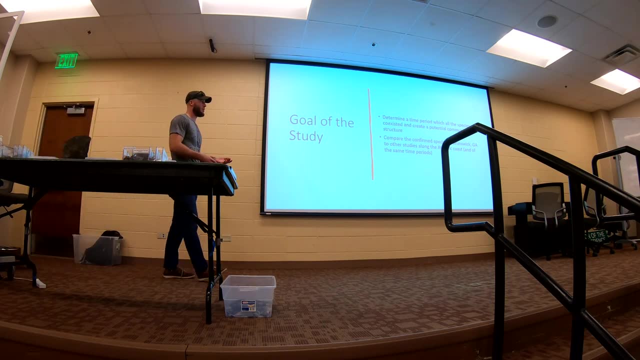 and figure out how far they were digging into each fossil bed and which ones they were digging into. So my goal of the study was to determine a time period in which all species coexisted and then create a potential community structure. I also wanted to compare my confirmed species. 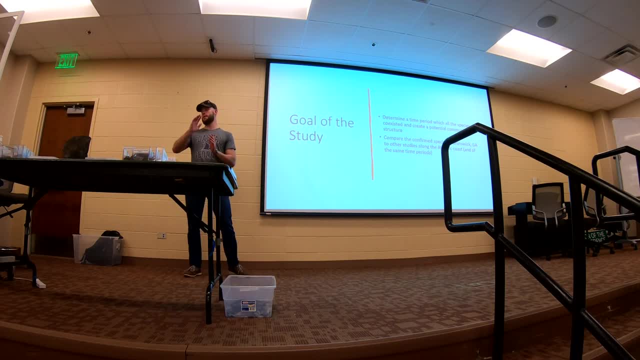 with other studies that may have been done in Brunswick, Georgia or along the Atlantic coast. So after about 14 months of collecting and about 400 hours of field time, I found 5,127 teeth, of which 4,981 of them I could identify. 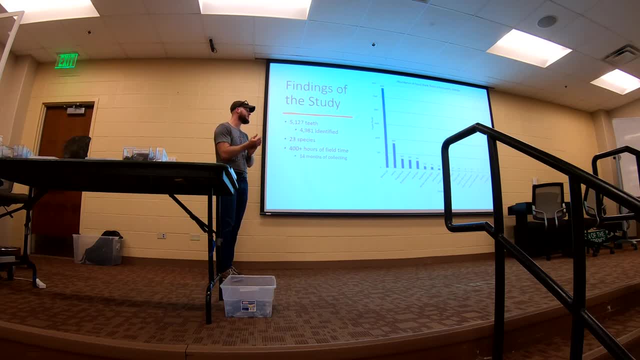 In total, I found 23 species and this kind of shows the relative abundance of each And you can see that the Megalodon was actually the sixth most prevalent species in my study And it far outcompetes the Great White. I only had 18 Great White teeth. 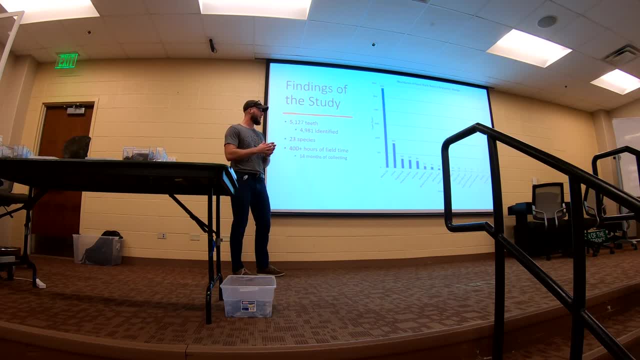 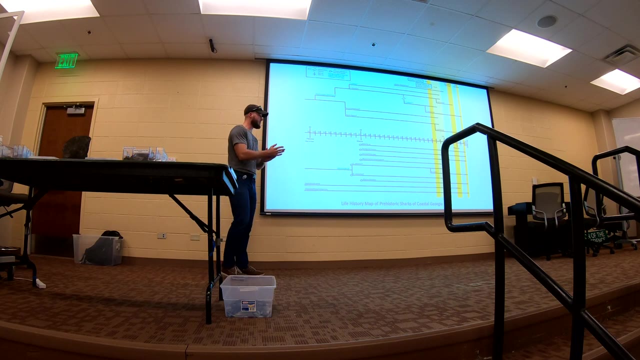 and 113 Megalodon teeth, So that poses questions as to why the Megalodon was so prevalent at the time. So I wanted to answer more and more questions as I started to get more data. So this is a life history map that myself and Professor Clark created. 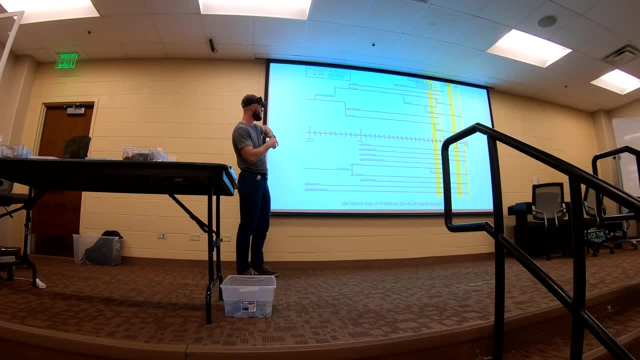 And so this is the life history of all of the species that I have, And each number here is millions of years ago, So we have 34 million years ago, all the way going down to present day, And so these are all the species that I have. 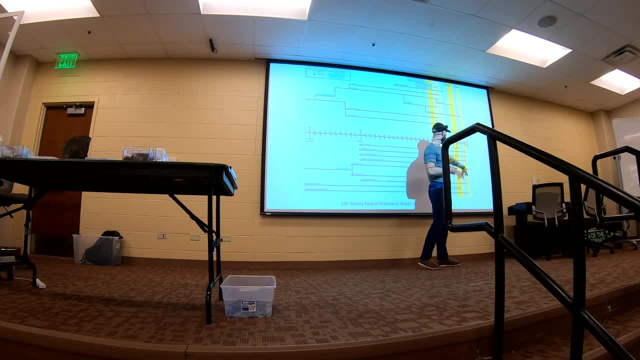 And these are the fossil formations that are being dredged into by the US Army Corps of Engineers, And so you can see their ages. And right here, in this time period, all of my species coexist, So that gives me room to start creating. 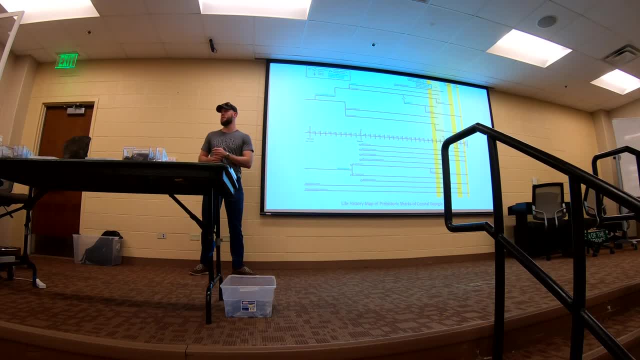 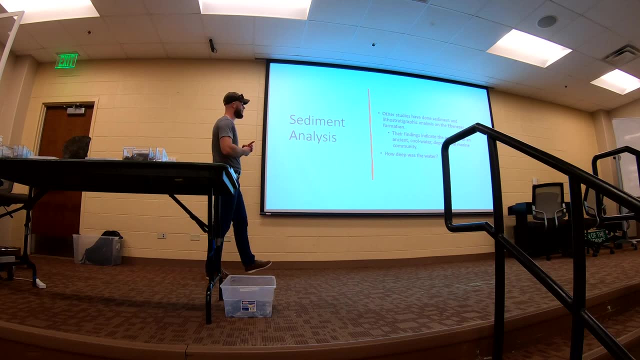 a potential community structure for that time period from around 8 to 3 million years ago. So I found some studies that did some sediment analysis of that fossil formation, which is called the Ebenezer Formation, And their findings indicate the presence of an ancient cool water depositional marine community. 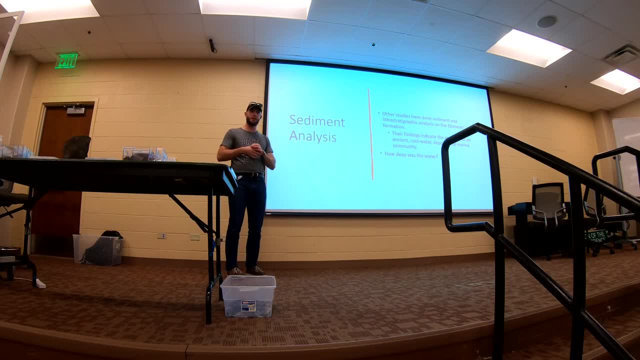 So I knew I was on the right track. I knew the area that I was working with did have sharks in it, And so the next part: I wanted to figure out how deep was the water. Sediment analysis can only do so much. 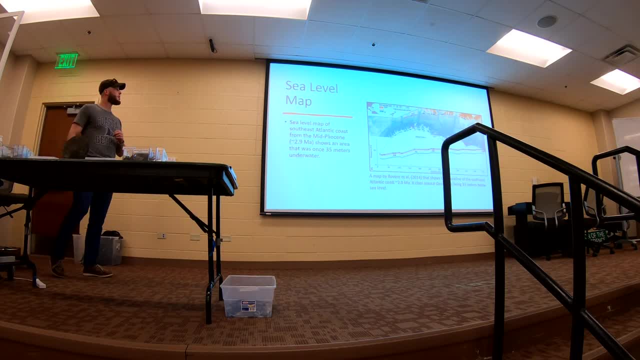 and it doesn't really answer how deep the water was at the time. So I was able to find a sea level map of the Atlantic coast from the mid-Pliocene, so around 3 million years ago, And it shows that the area was once. 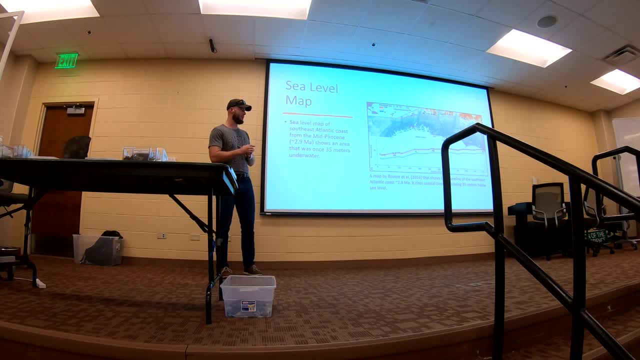 35 meters underwater around the time of the Ebenezer Formation. So now we kind of have starting to paint a picture of what this area looked like, where all these sharks existed at one time, And so it was determined in a couple other studies. 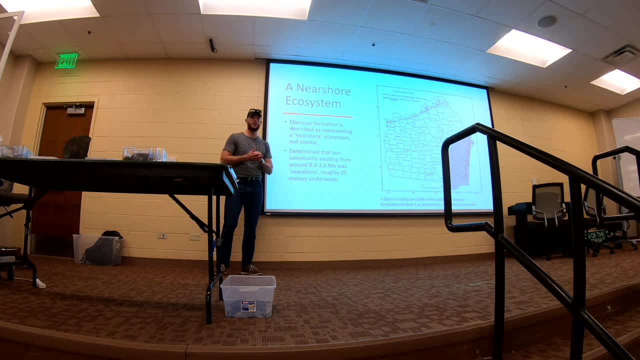 that the Ebenezer Formation represents a near-shore ecosystem, not coastal, And so from there, there's lots of different definitions of near-shore if you talk to different people. So we are saying that a near-shore ecosystem is what we're working with when we're talking. 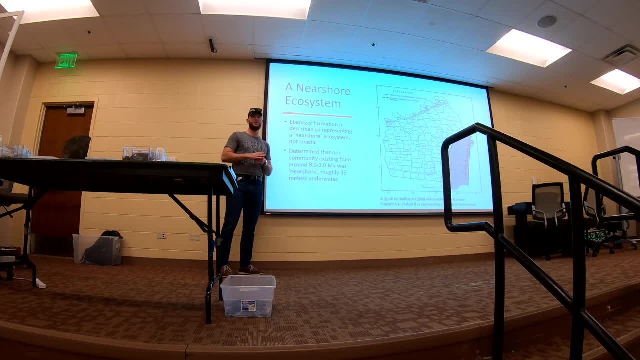 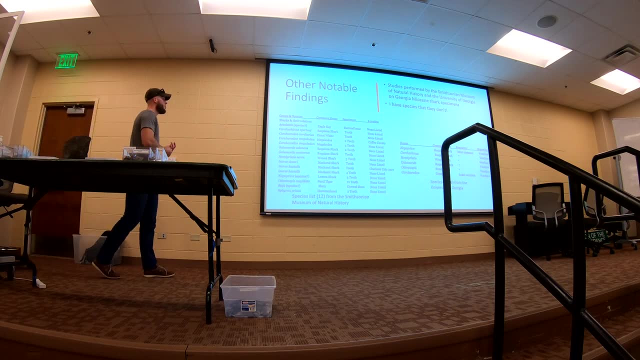 about the Ebenezer Formation And it was around 35 meters underwater. Okay, so some other notable findings. I mentioned that I wanted to compare my species list to other ones that have been done in coastal Georgia And I found two, One done by the Smithsonian Museum of Natural History. 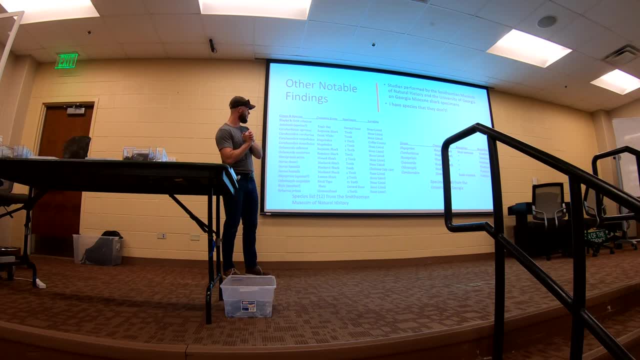 and another by UGA And the Smithsonian. this is their list and they have 12 species, And the species list from the University of Georgia has six species And I have 23.. So I would love to. I'm going to contact them pretty soon. 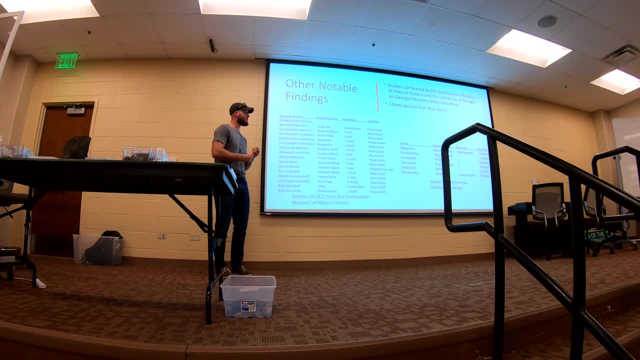 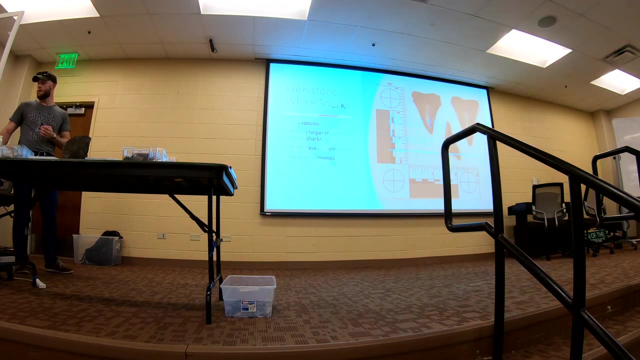 and send them my findings to see what they think about it. see if I, you know, would be of any contribution to the current understanding of shark paleontology in coastal Georgia during the time. So a little bit about the species, just a few of them. 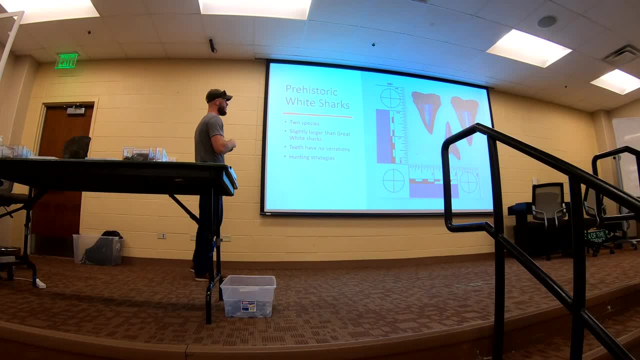 The prehistoric white sharks. This was a pretty common group at the time and they far outnumbered the great white shark. We have two species. They were slightly larger than great white sharks. They could get up to about 30 feet in length. 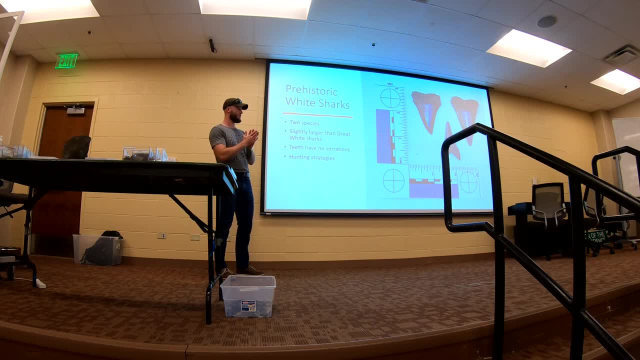 Their teeth have no serrations. The great white did develop serrations over time And hunting strategies. Basically, we think that the extinct white sharks had the same exact hunting strategies as the great white, Where you might have seen like Nat Geo or something like that. 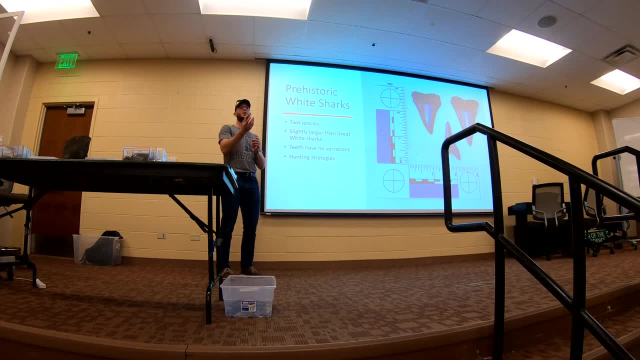 when they hunt marine mammals such as seals, they come from the underside as a supposed sneak attack or, more commonly understood, they come from underneath to hit the vital organs and basically it's a quick kill so that the great white doesn't have to use too much energy. 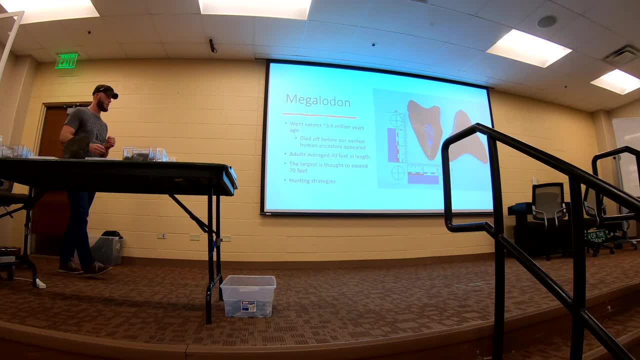 to get their food. The megalodon, on the other hand, its hunting strategy was a little bit different. They were looking at whale bones and they were figuring out that megalodon based on the tooth marks inside the whale bones. megalodon were striking from the side. 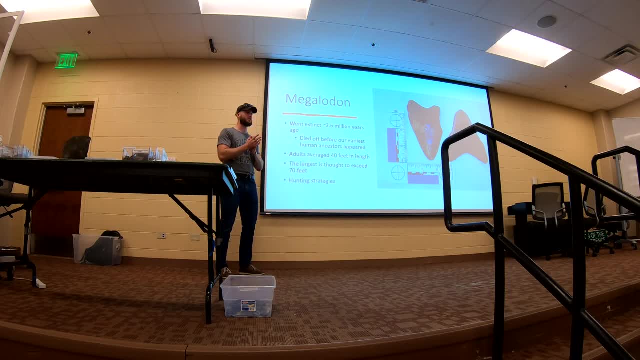 And they hypothesized that the megalodon would strike from the side to puncture the lungs and then the lungs of the of the marine mammal would fill up with water, they would drown and then they would go eat them. So they were a little bit more gnarly than the great whites. 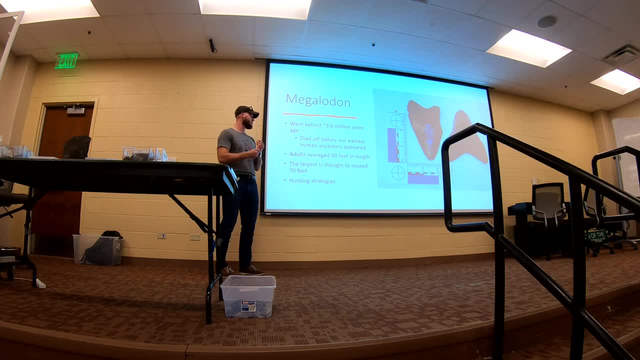 Megalodon did go extinct around 3.6 million years ago, So they died off before our earliest human ancestors appeared. That was kind of a relief. Adults averaged about 40 feet in length. The biggest one is thought to have exceeded 70 feet. 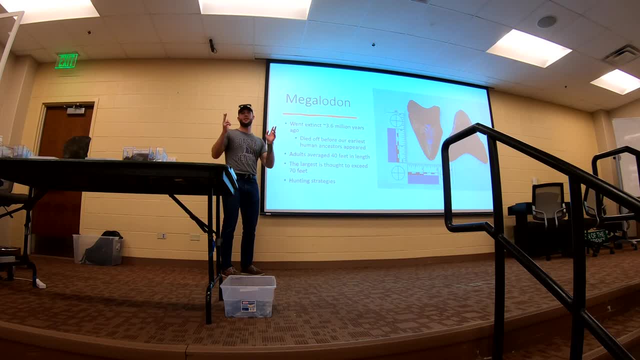 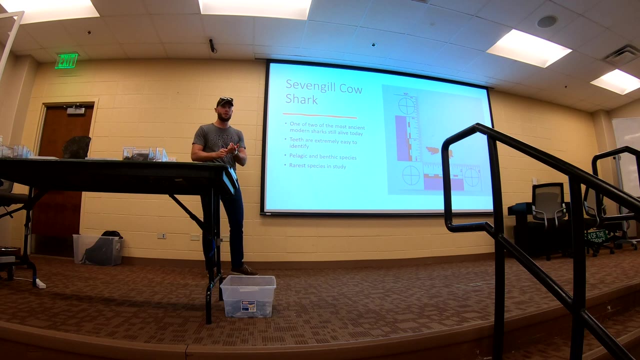 So if you've ever seen the meg, that size is about right for what the largest megalodon is, Sorry. And so the rarest species in my study was the seven-gilled cow shark. It's one of the most ancient sharks that are still alive today. 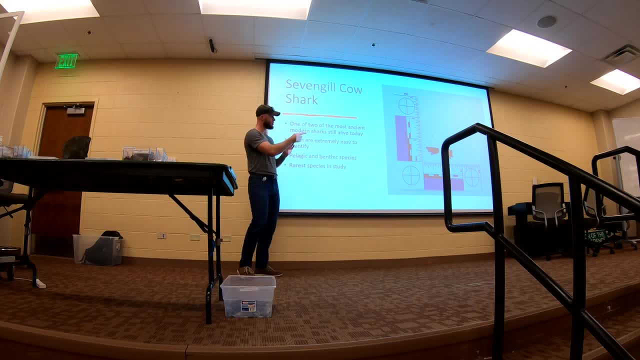 And their teeth are extremely easy to identify. Each of those is just one tooth. The one on the right is just actually a fragment of the tooth. You can see that these two are right there, like those right there, And so their teeth are. 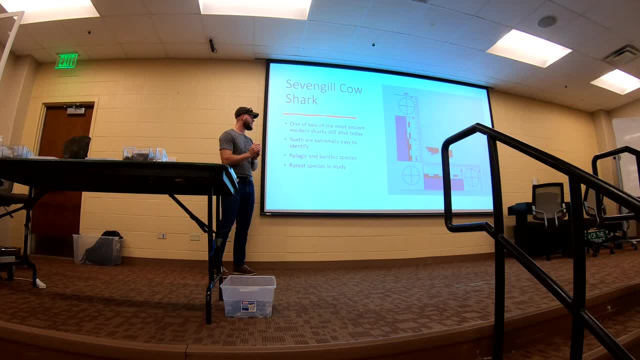 really rare. I only had two out of over 5,000.. And so it was interesting to know why they were here at the time, because they're known as a pelagic and benthic species. So they're on the bottom floor, out in the deep ocean. 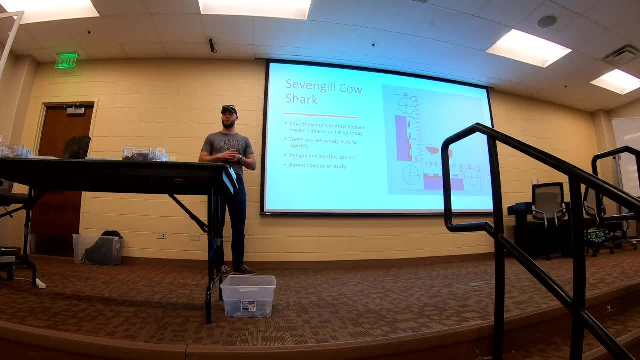 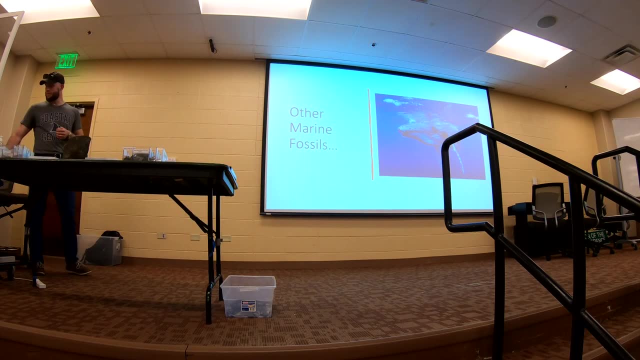 And so why would they be in a near shore ecosystem? So that raises some more questions for me to want to answer. So some other marine fossils that I found: We found some dugong and manatee rib bones, So you're probably familiar with manatees. 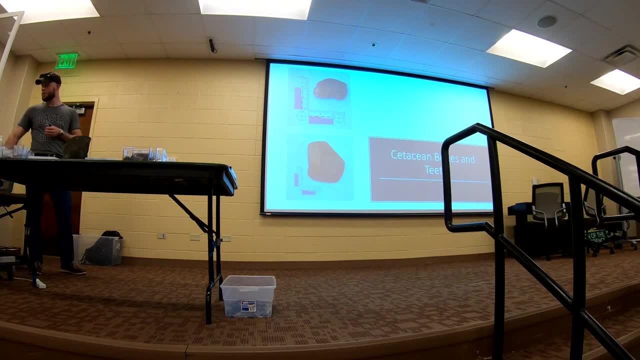 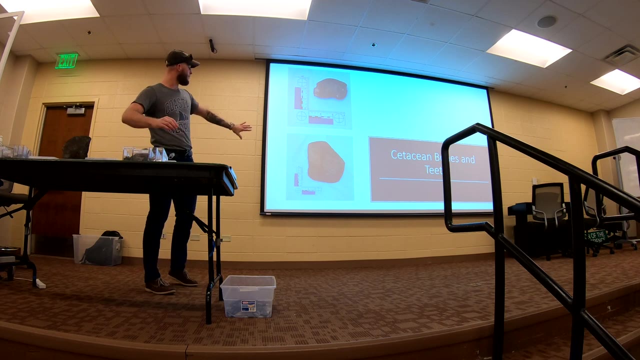 We found lots of rib bones all along the island. We also found some cetacean bones and teeth. There on the top is a whale ear bone right here, So it's pretty big. They have big ears And their vertebrae right here. it's just half of one, but it's around eight pounds, So it's very big And this would have been the prime food for megalodon. We have odontocete teeth, which are the toothed whales, So we weren't able to narrow them down to specific genus and species. 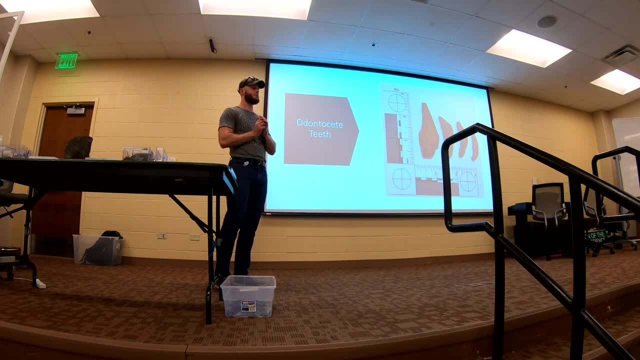 Because they're dredging. we were working with three different fossil formations And to properly identify a fossil, you need to know which fossil formation it comes from And since they're being dredged and stirred up, I don't know which of the three that they're coming from. 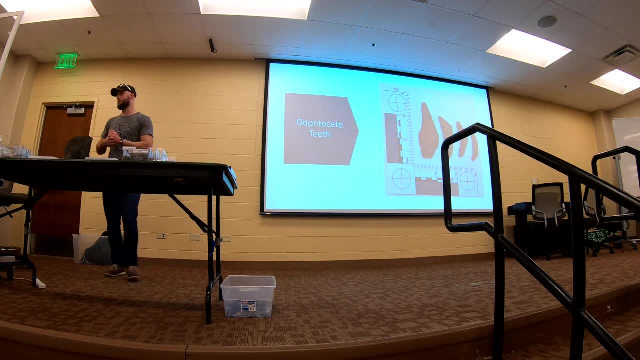 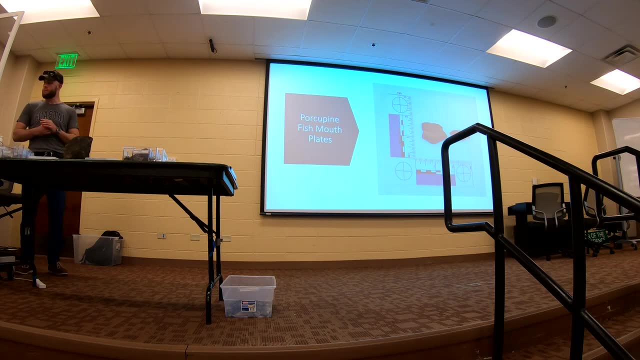 So we're not able to properly ID a lot of these marine mammal fossils. We also have stingray spines and mouthplates, Porcupine fish mouthplates. We have one sawfish tooth. I found one in the entirety of the study. 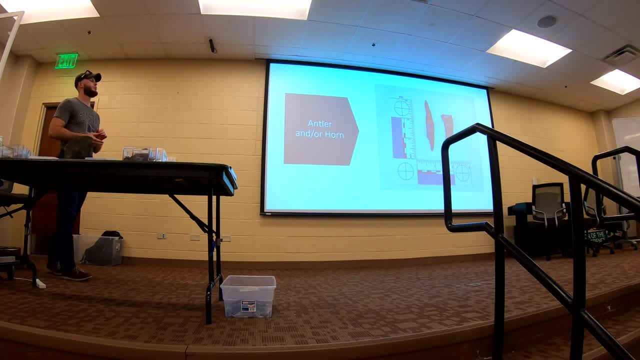 We have some sort of antler or horn from a terrestrial species during the Pleistocene, So from probably around 10,000 to 20,000 years ago. We aren't able to ID it. We're trying to do that right now. 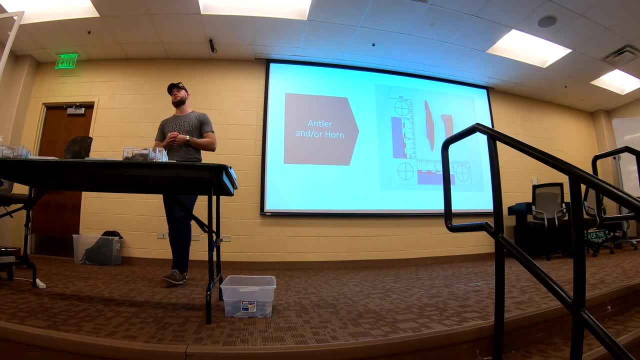 But those two specimens we believe are antlers or horns of some kind. We have alligator and crocodile teeth. On the far left is an alligator tooth And the two on the right, the middle and the right are alligator teeth. 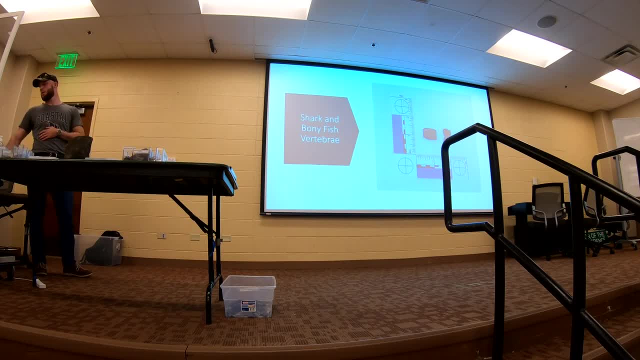 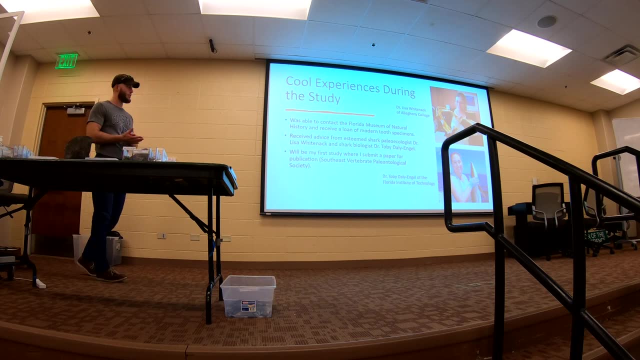 We have some barracuda teeth. We also have, as you've seen before, shark and bony fish vertebrae, So some cool experiences during the study. As I said before, I was able to contact the Florida Museum of Natural History. 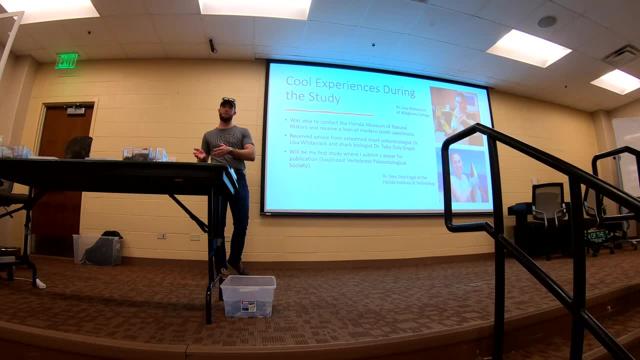 and receive a loan of modern tooth specimens to compare to my fossil. They were super helpful and encouraging in my study And they have constantly been reaching out to me to know more about my study. They want me to send them my paper when I get it finished. 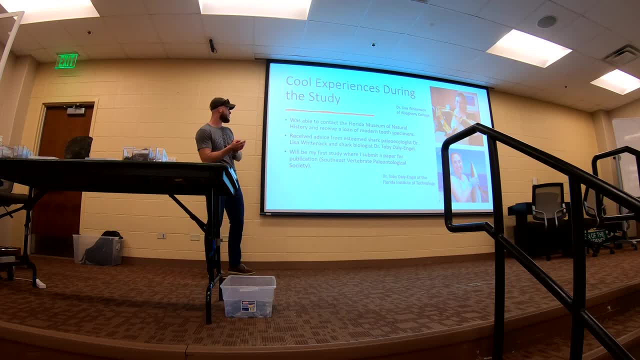 I received advice from a shark paleoecologist, Dr Lisa Whitenack, and shark biologist Dr Toby Daly-Engel. Some of you might be familiar with Dr Daly-Engel. She's really nice. She's from the Florida Institute of Technology. 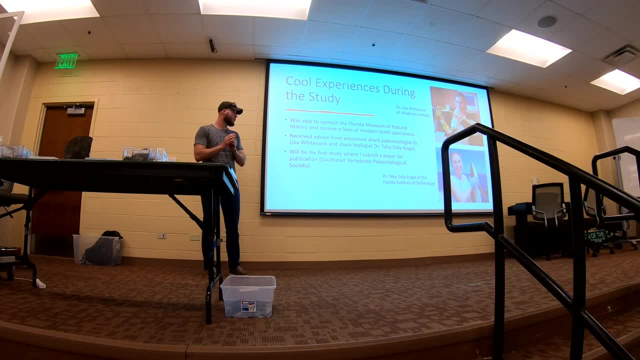 And this will be the last time. this will be the first study where I submit a paper for publication. I really hope to send this to the Southeast Vertebrate Paleontological Society to get it published. So that's the goal now Over the next couple of weeks. 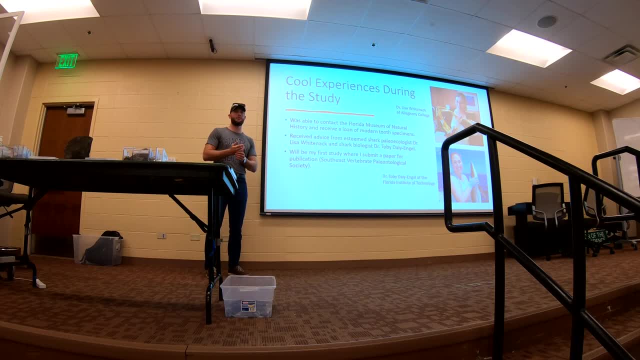 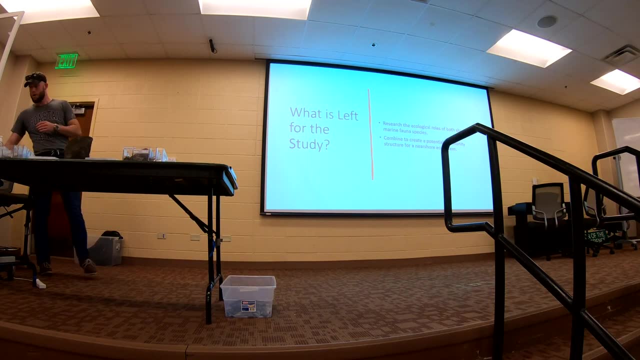 me and Professor Clark are going to be working on fine-tuning my paper for publication. Alright, so what's left for the study? So this is just part one of the study. Part two will be researching the ecological roles of both shark and marine fauna species. 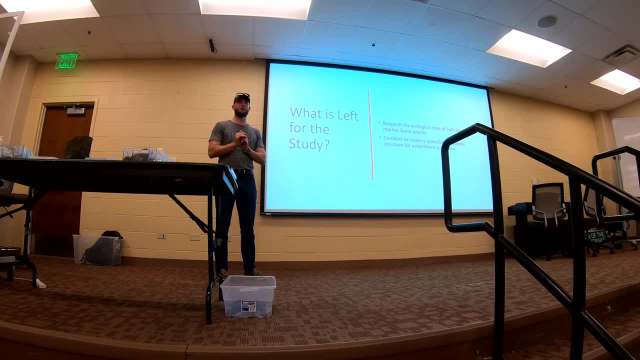 During that time so I can create a potential community structure. So I'll be won't be anymore collecting, but I'll be really trying to figure out the ecological roles so I can really better paint a picture of what this place looked like around eight to three million years ago. 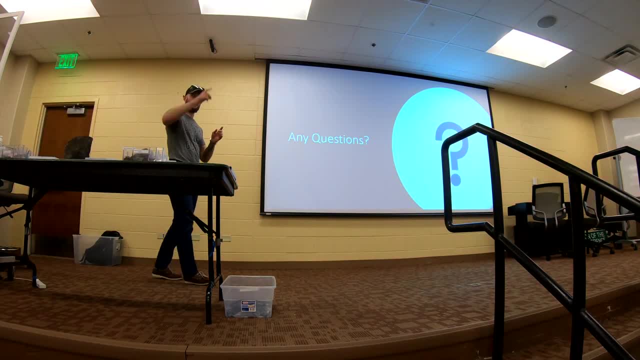 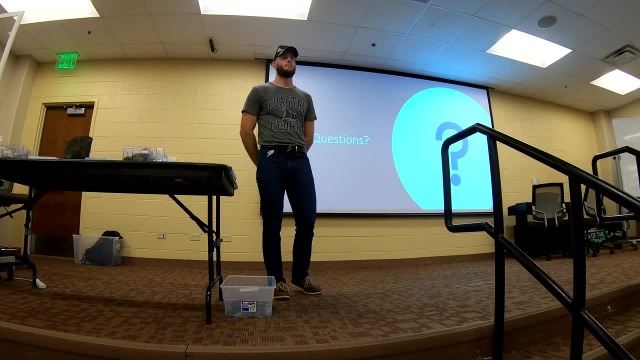 Any questions. Morgan, I was just like kind of thinking as I was listening and you know how, between like Jekyll and St Simons, a bunch of sharks, that's like I don't know what is it like? the third biggest breeding ground? 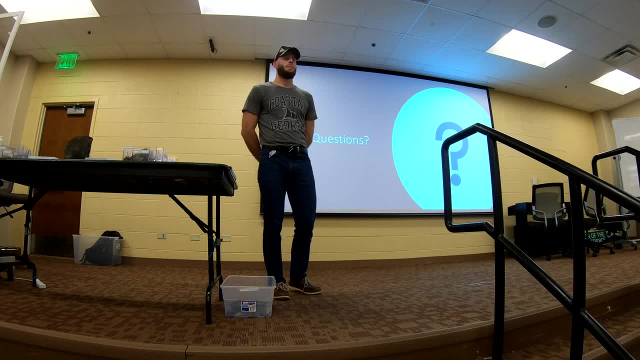 Yeah, it is a breeding ground. yes, So I was just thinking like, because there was a bunch of different sharks that you found and that area like 35 meters is I mean, like you said, it's kind of like a deeper, like. but it's not like they couldn't have lived there their whole life. You know sharks would migrate or whatever, But would you think that maybe, like certain megalodon species and stuff like that, could have been coming there even back then? because they tend to repeat patterns to breed maybe, Yeah, I think megalodon were. definitely they were. they've been found in areas that were once coastal, So they were found in areas that were super shallow, like way more shallow than 35 meters deep. 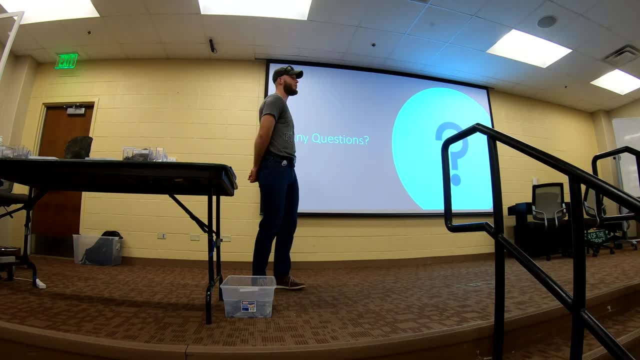 So they just like great whites. great whites like the coast, They like the open ocean, They like everything. So megalodon really didn't care where they were, They just wanted where food was, And so the presence of marine fauna really indicates that this could have been. 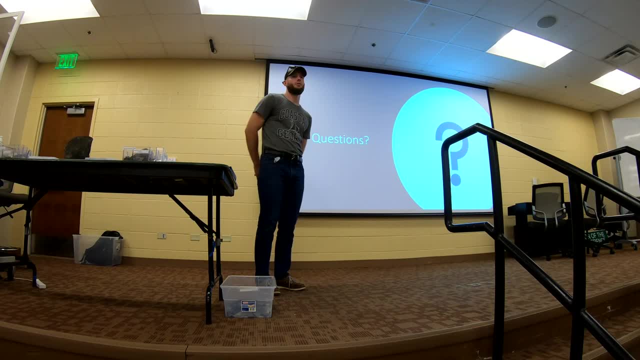 a megalodon nursery, because I have a lot of juvenile megtips. So they could have, you know, been smaller and they could have been in more shallow areas at the time. Anything else, Mr Lucas. So if the white sharks were slightly bigger, 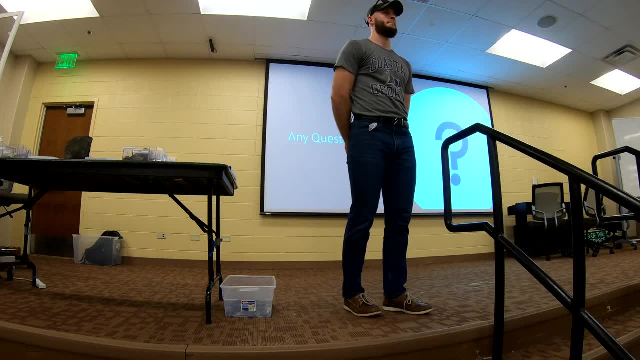 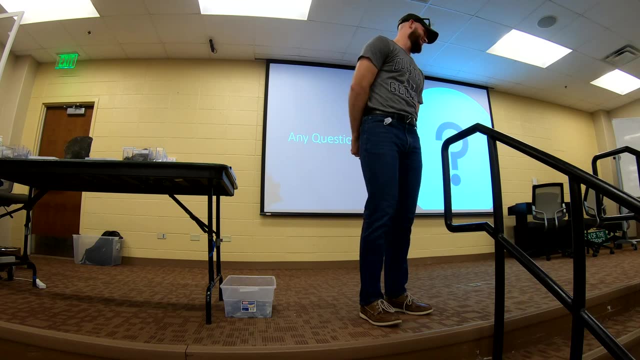 than the great white sharks. why are the great white sharks called the great whites? Why are they the great whites? That I don't know. I personally like the extinct white shark's teeth better than the great whites, So in my opinion they're kind of like the great whites. 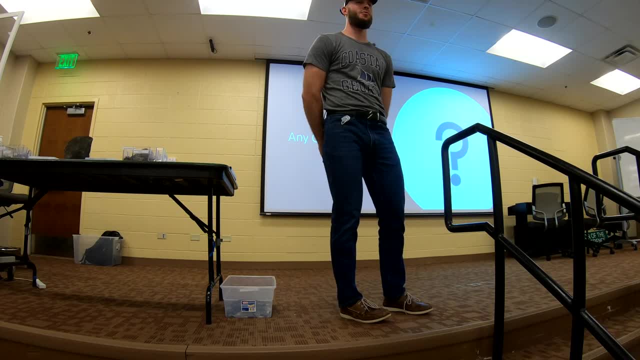 But I don't know why they're called great whites. I'm sure the extinct white sharks were discovered after the great white sharks. So if we called them the great whites, then we probably realize: oh crap, we probably should have called them the great whites. 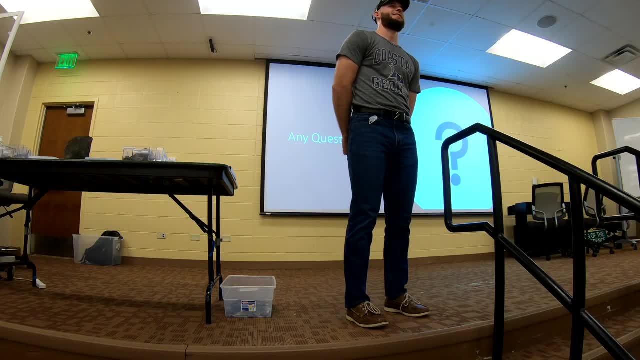 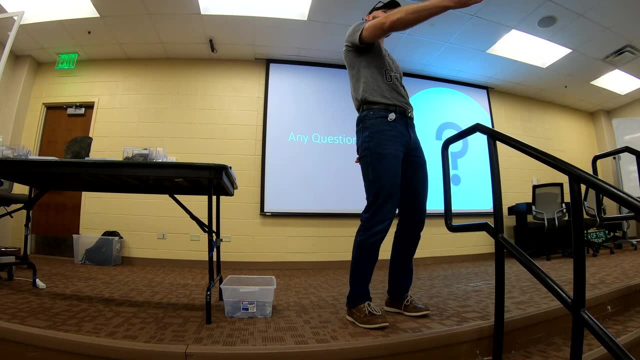 You should have done like you would with birds and just called it a greater white shark. Yes, That would have been nice, But instead we have narrow white shark. Oh, we have. one of them is called the giant white shark, And I do have. 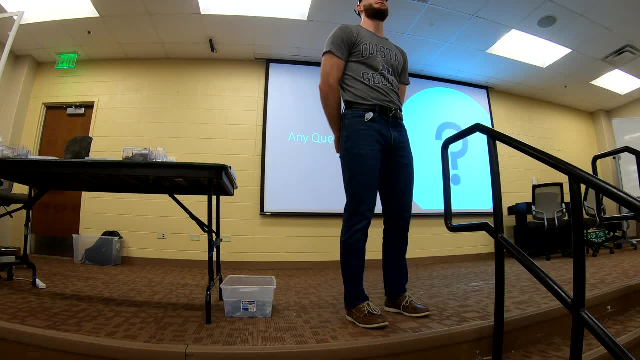 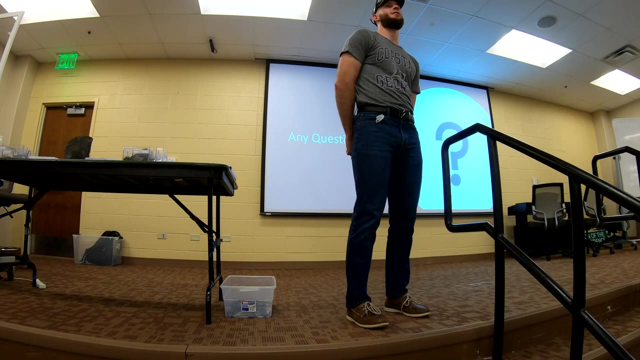 and I do have a species of that. So, Chandler, What's one of the major things you learned from this experience? Hmm, One that the DOT, the Department of Transportation is mean And they don't want me going to their sites. 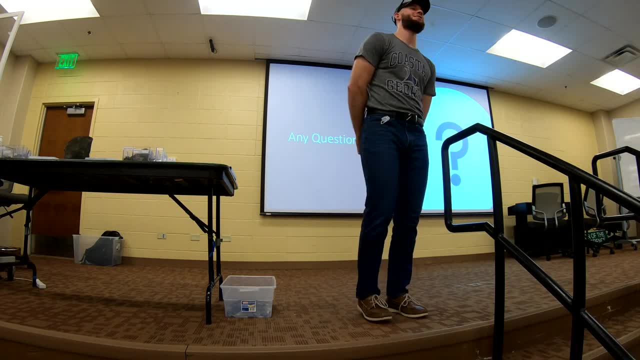 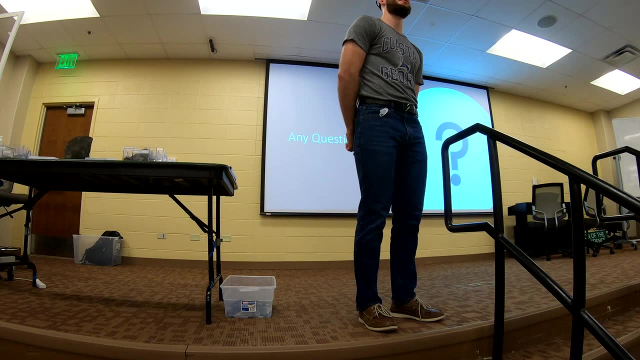 where they dump all their stuff And two other than the DOT. people are really receptive to people who are trying to do research, especially for the first time. Everyone that I reached out to- paleontologists, paleoecologists, universities. 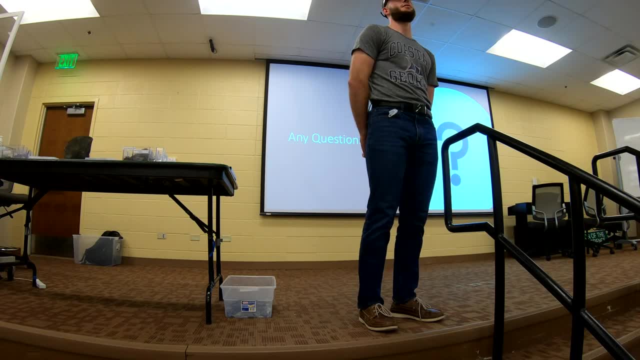 museums. they were all super helpful, super responsive, So that was really encouraging to me. I was really really happy to get like quick responses from them, So I was really impressed by the fact that they were so, so helpful. So, yes, 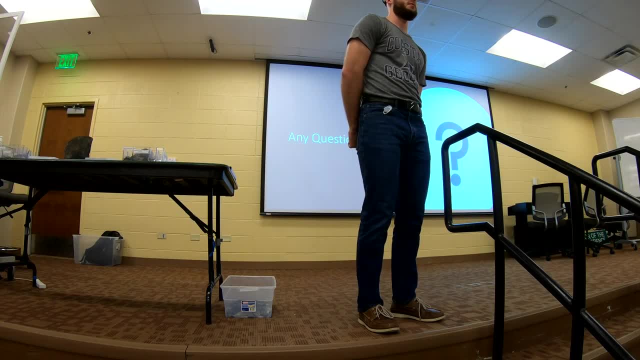 Where did you start? where did your friends at the time tell you to start searching museums? They all they said, and, for the most part, the few people that know about the location you know. you're not allowed to say where it is. 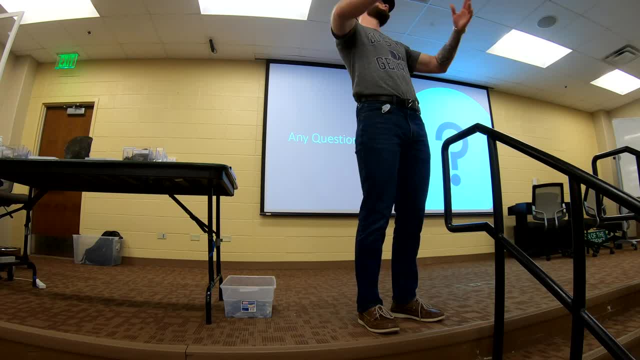 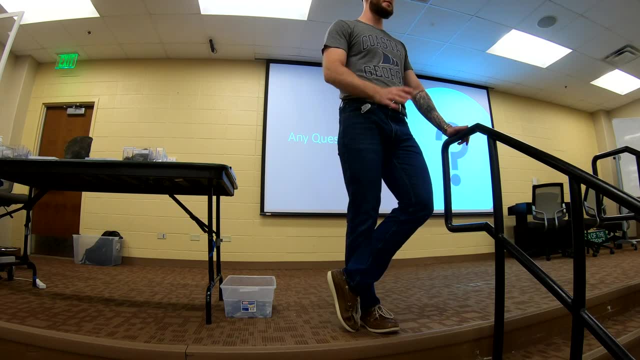 just for just because it's. they don't want people everyone coming there, And it's only accessible by boat as well. You can't walk to it or anything- And so they found it and they. the only detail that they would give me is: 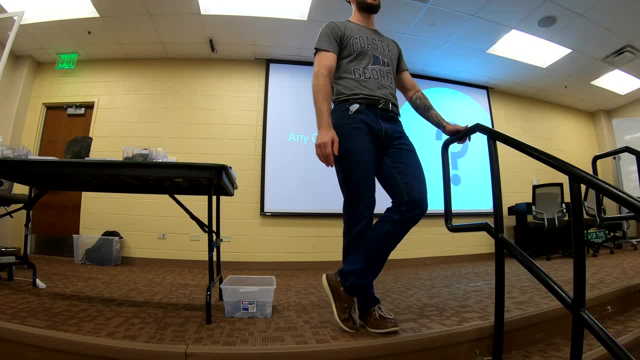 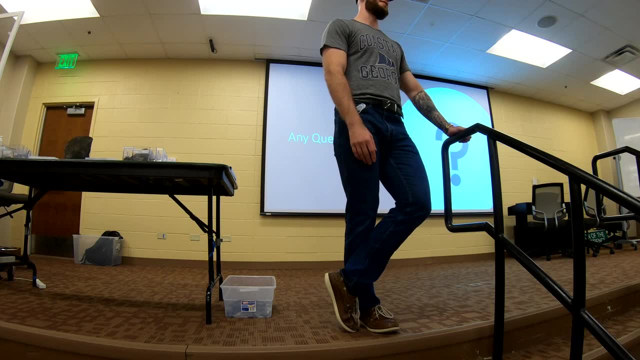 you need to get off at the Sidney Lanier Bridge. There's a boat ramp underneath it, And so they said: get off there and good luck. So that's all I had to go off of. That's the fun of it, So yeah. 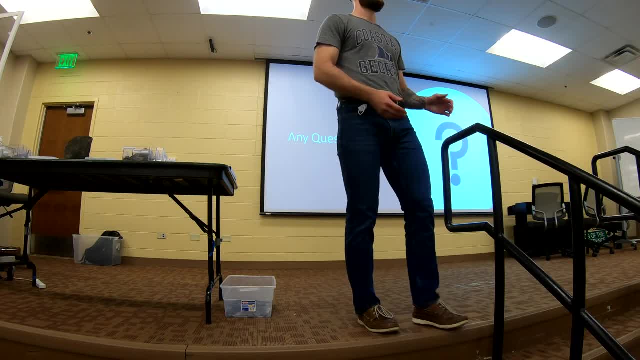 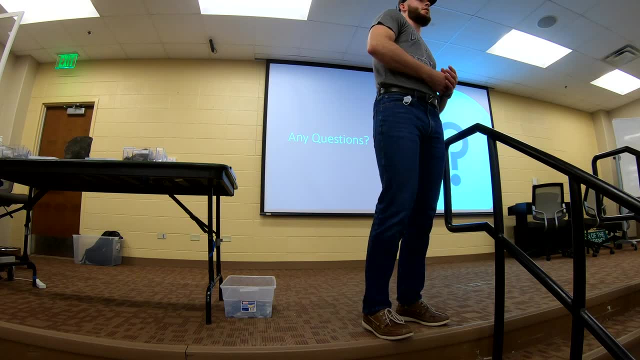 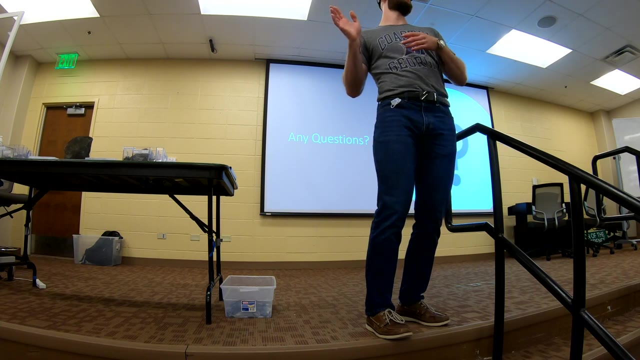 Yes. Can you say something about how they survived four out of five mass extinctions? Can you explain why four out of five Versus like all five? or There was a mass extinction before? Yeah, So like there was a mass extinction where sharks didn't exist yet. 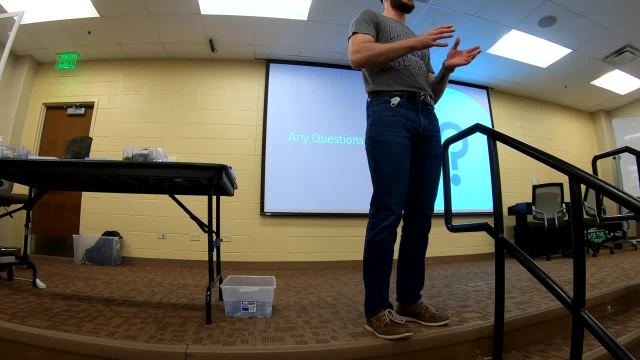 And so so, since they've, since they've came about every mass extinction that has come along, they've been able to persist. So So, basically, they survived out of the human sky. Yeah, We're, we're, we're giving the other ones a run for its money. 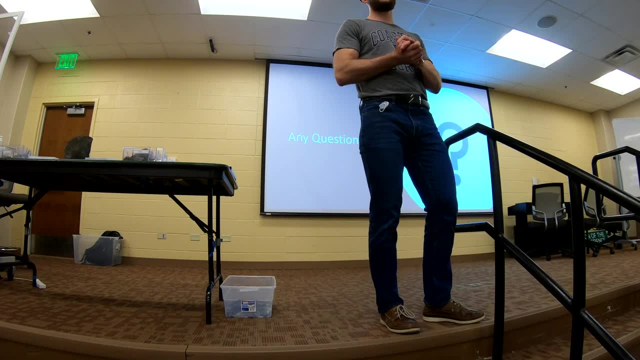 Anything else? Yes, Well, you were talking about the serrations of the teeth. Um, what did you say about? like the great white and the other white shark? What about them? specifically About the serrations. Yeah, So let me go to them so we can see. 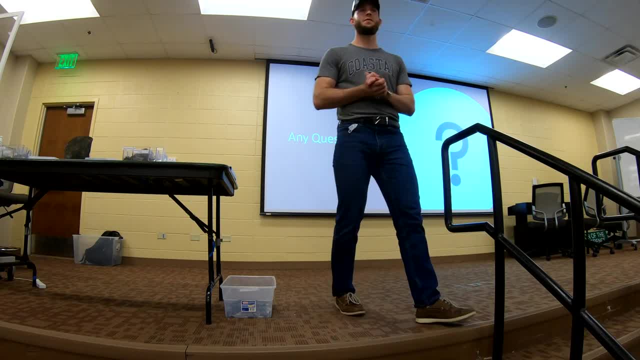 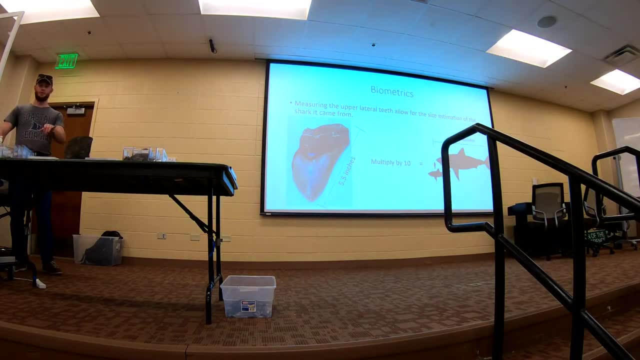 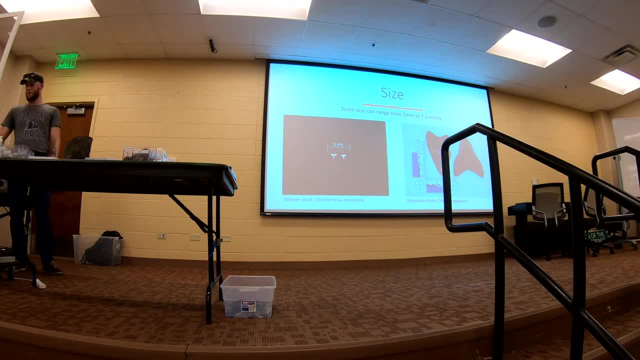 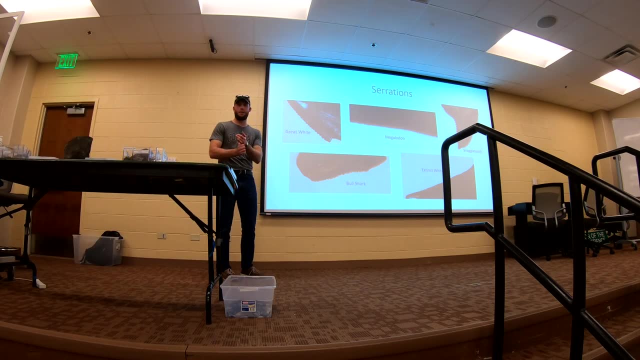 I'm, I'm, I'm, I'm more than happy for you guys to to look at them up close. Um so serrations are? they can be classified as different things. They can be classified as simple, complex. 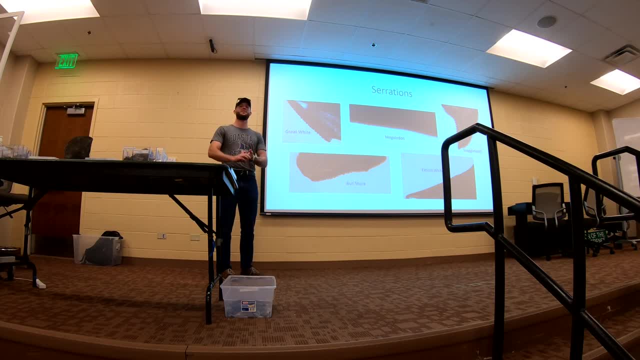 coarse, fine, So, uh, running through them again. the megalodon serrations are described as small and fine. Um, each tooth, each serration is really similar to the one next to it And they're pretty small compared to the overall. 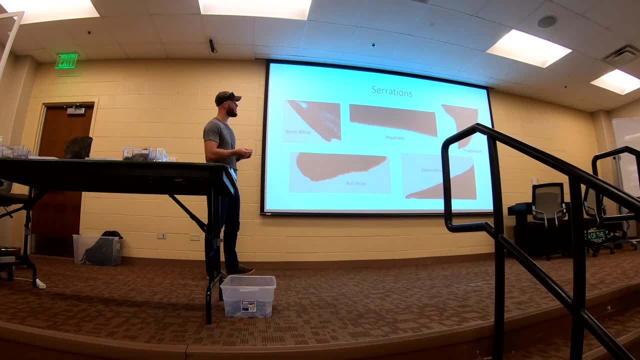 um size of the tooth. Great white serrations are a bit bigger Um and and and and and and bigger in um in proportion to to the tooth size And you can see here they're kind of irregular looking. 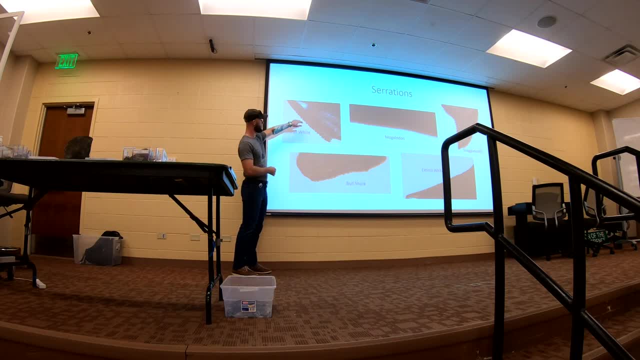 and they're a little bit um spaced out And they form these things that no other species forms, called complex serrations. We're two serrations, um basically fused. They can't figure out if it's one serration. that kinda splits off. 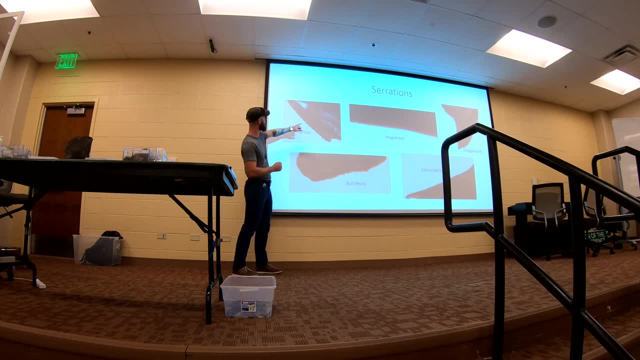 or if its two serrations that almost fuse together. But you can kinda see examples here and here and here Where they, where it looks like there's kinda two that are just stuck together And they so those are called complex serrations, kind of serrations on top of serrations. 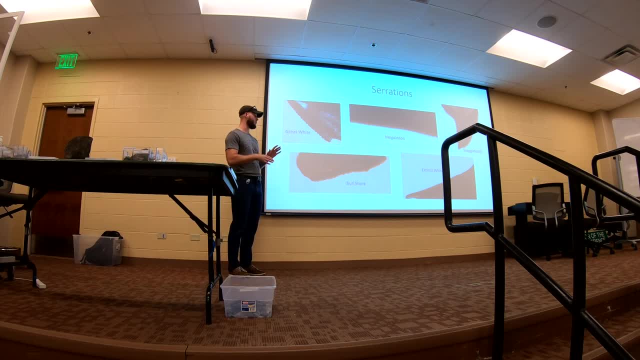 and in a bull shark serrations. you know those are all irregular and would probably give you a nasty cut, and others don't have serrations like the extinct white shark, and so it's really cool to see transitional species between the extinct white and the great white. there were species in between there where you 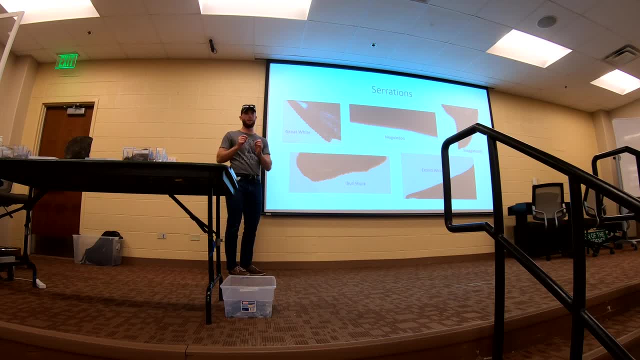 can start to see serrations starting to form, but they're not quite there yet. so it's pretty cool. and the snaggletooth sharks have just really pretty serrations. they're very big. it all just kind of depends on their diet, what they were specialized for at the time, anything else? 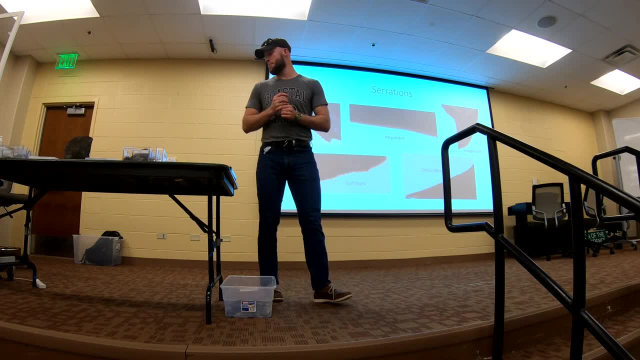 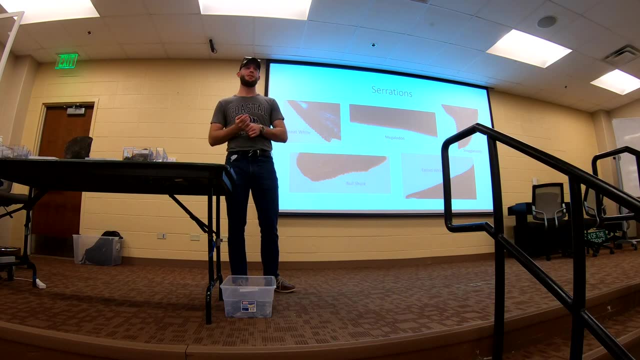 yeah, so when? so a little bit of history about megalodon teeth. when they first found them they thought they were the tips of dragon tongues. way back in the day, that's what they thought they were- dragon scales. and when someone was studying it he realized, hey, this looks a lot like a great white shark because 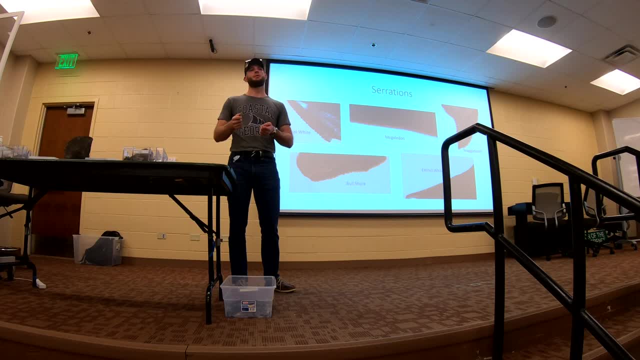 they already knew what a great white shark was at the time, and they knew what their teeth looked like. so they said, hey, this looks like a great white shark. this might be from a shark actually. so that's how they determined that it was indeed a shark tooth. over time they started to